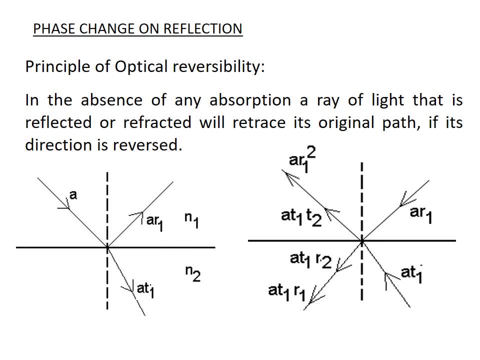 In the absence of any absorption of ray of light there is, that is reflected or refracted, trace its original path if its direction is reversed. What it is saying is, if the total ray, there is no loss of the amplitude taking place, then whether it is getting reflected, whether it 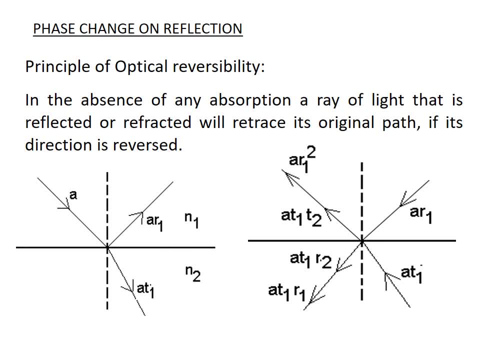 is getting reflected, or reflected or refracted, then it will retrace its original path. Let us just take two medium, n1 and n2, and the ray of amplitude. A Medium 1 has a reflective index of mu1. whatever you take n1 and n1 and second has n2.. The reflection coefficient: 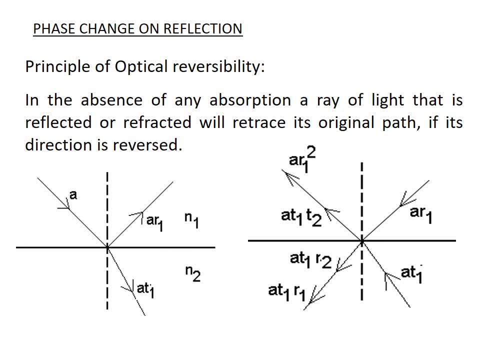 for medium 1 is r1. transmission coefficient for medium 1 is t2.. Similarly, for medium 2, we have reflection and transmission coefficient as r2 and t2.. Any ray that will fall on the surface or the boundary of n1 and n2, it will get reflected. 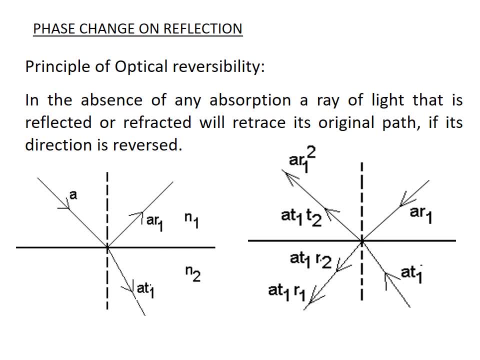 and transmitted. This division of the amplitude is utilized in the Newton's ring experiment that we will do later on. Let us just see: we will be retracing the reflected rays path and the transmitted rays path, For example. look at the second picture. or let us, coming back to the first picture, the amplitude of A, the amplitude of A it. 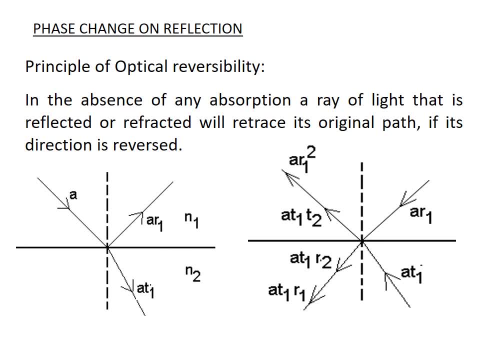 is getting reflected, The amplitude becomes ar1 and, as it gets transmitted, its amplitude becomes at1, because it is getting reflected and transmitted from the first medium. Now, if you want to retrace the path of ar1 and at1, what we will do is to come to the 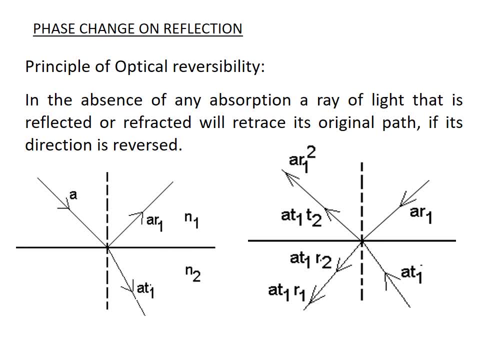 look at the second picture: ar1. it is getting transmitted, Therefore ar1.r1, and it is getting. sorry, it is getting reflected and it becomes ar1, r1. that is, ar1, square, and it is getting transmitted. it becomes ar1 and t1, this one. Now look at: 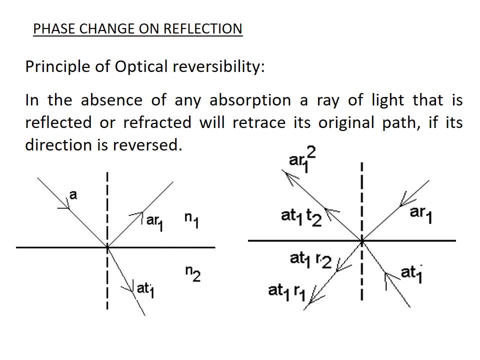 the transmitted ray, part at1 is getting reflected, it becomes at1- r2, since it is getting reflected on the second medium and it getting transmitted, it becomes a t1- t2. now i will be, i will be saying talking in terms of quadrant. just just, let's just look here: first quadrant, second quadrant, third quadrant, and 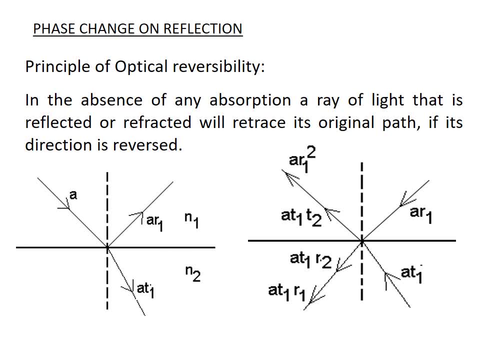 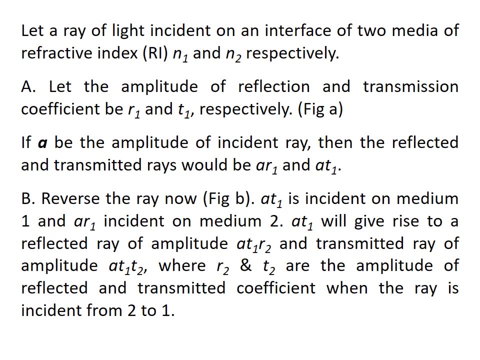 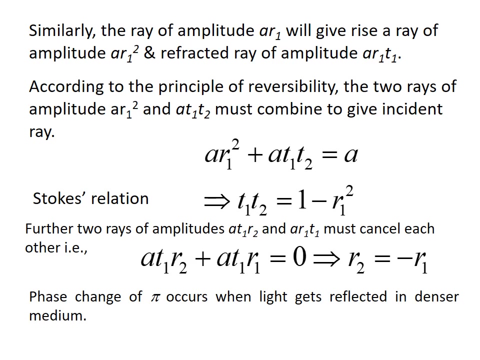 fourth quadrant. we will be matching the first and the second figure in the second quadrant. this is what we have discussed: the two media, n1 and n2, and the amplitude are getting splitted or divided as a t1, ar1 and so on. not all in the second quadrant. comparing: 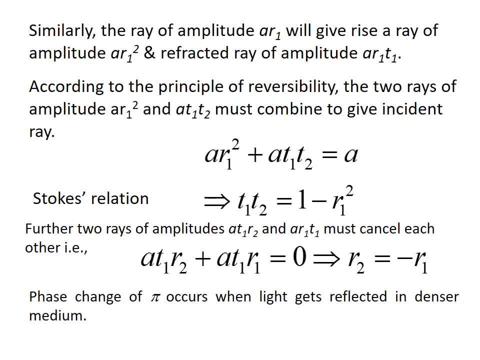 it the two figures. that is, we go again and we go to. we get the equation first equation as ai gets sp night now. this is the first equation, this is the second equation. i am using uh plus and minus and this is the figure i and we use two. we get the first one can't. be coll 나가etal. now, in the second quadrant, all factorsi will be organization어를 here. second quadrant, all different styles, all different values, all of it the right things that myомat ph on nine it can be you know other all it can be. one it can be Gonzalez abender. 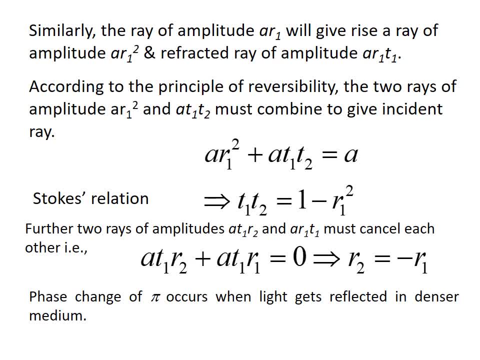 R1 square plus A T1. T2 equals to A and just by simplifying we get a stoke relation. equals to T1. T2 equals to 1 minus R1 square Further, for the third quadrant, the equation is: A T1- R2 plus A T1 R1 equals to 0, which. 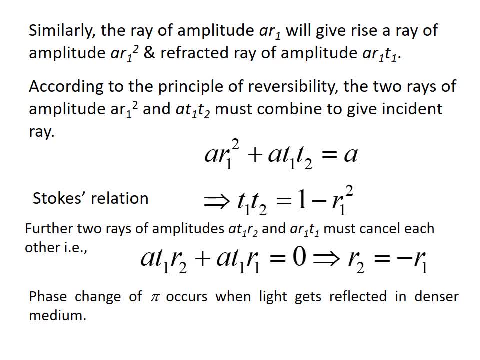 implies that R2 equals to R1 and at the reflectance. when the reflection takes place, then a phase change of I is occurring and the lights get reflected in the denser medium. This is only possible when light is going from the rarer to the denser medium, that is. 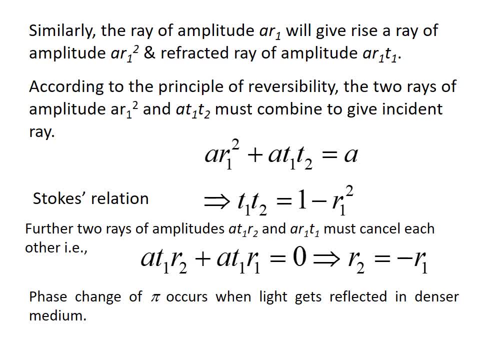 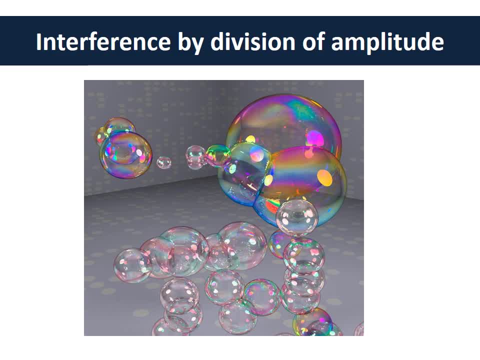 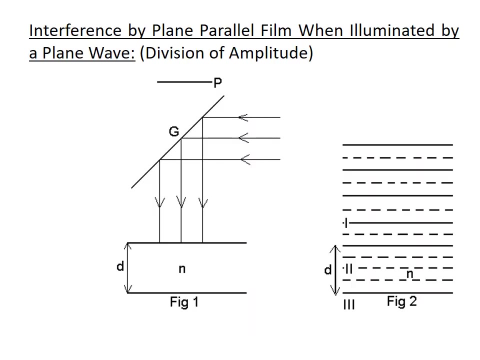 refractive index of N2 is greater than N1.. As the phase changes, R2 equals R1. When the reflection takes place from the rarer to the denser medium. let's just see the interference by the division of amplitude And the interference by the plane. parallel film, when illuminated by a plane wave, looks like: 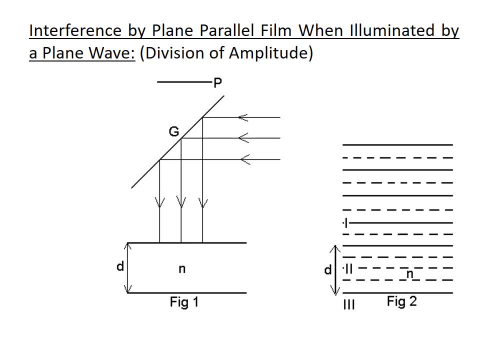 We have the plane waves falling on a partially reflecting mirror surface, The reflected waves. they fall normally on the material. This material has the upper and the lower surface and is of the refractive index n, Having thickness mol d. the reflected wave from the upper surface and the lower surface. they interfere and form the interference pattern. 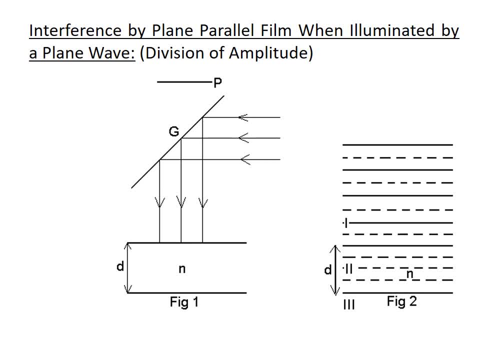 Since the refractive index of the material is of the lower surface, it is of the upper surface. If the material n is greater than the refractive index of the material n of the air that is here, then the wavelength will be different inside here. 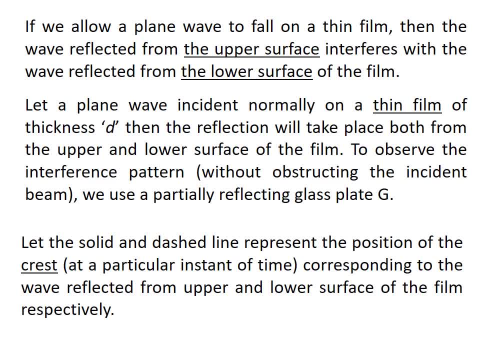 If we allow a plane wave to fall on the thin film, then the wave reflected from the upper and the lower surface of the film. they interfere and form the interference pattern. For that let us take a plane wave which incidents normally on a thin film of thickness mol d and refractive index mol n. 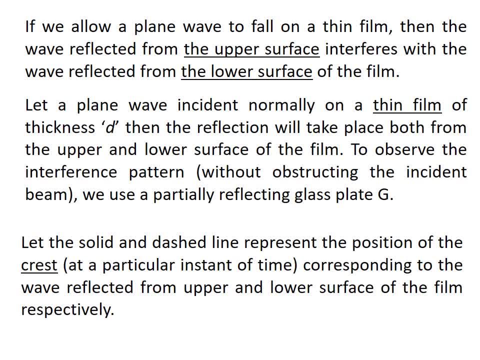 Then the reflection will take place from both the surfaces, that is, upper and the lower surface of the film. To observe the interference pattern we use a partially reflecting glass plate. G In figure 2, the solid and the dashed line. they represent the position of the crest at a particular instant of time, corresponding to the wave reflected. 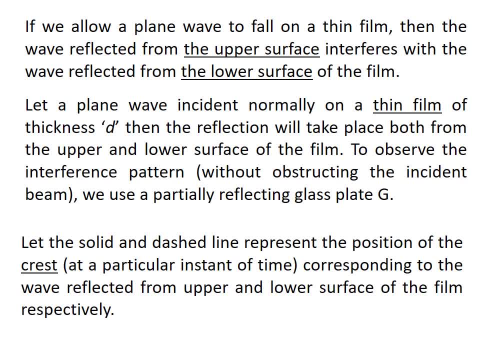 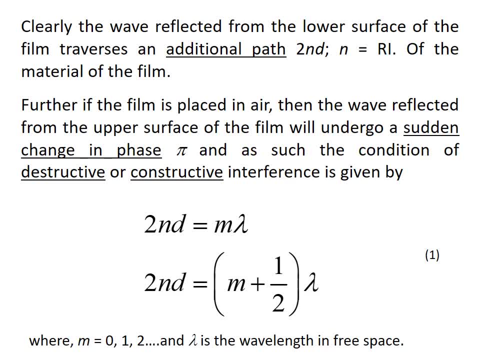 Like this. it is characteristic even for the order. this particle gets reflected in an instant. Similarly, we have a individual wave, entrepreneurs. we see here the wave is not reflected from the upper and the lower surface of the film. The wave reflected from the lower surface of the film will traverse an additional path. AmaH Raghu. 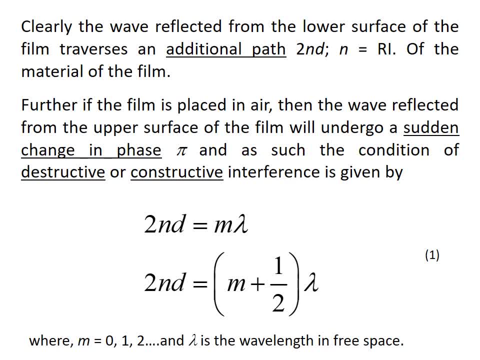 or as we saw in figure 1, On the째 we see the waves from the lower surface of the film. they will traverse an additional pathаг lesson: Gd �mägłego So se example Gd bmg. from there, The reflected beam from the lower surface will travel additional distance of 2N taki bmg, gd 3Mpa From the surface of the film. the indicated itself Ndb will thenverse from the lower surface of the film and hence another additional distance is appeared. if an additional extra distance is occurred, 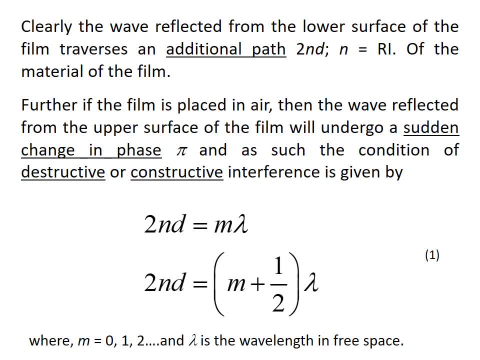 where n is my refractive index of the medium or the material of the film. therefore, the additional part of the part difference between the two reflected films which will interfere and form interference pattern is 2nd, for simplification here. further, if the film is placed in air, 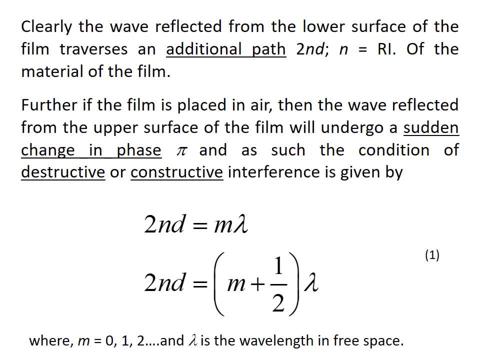 then the wave reflected from the upper surface of the film will undergo a sudden change of change in phase, as discussed before. if the wave travels from the denser rarer to the denser medium, then the change of phase pi occurs. then the conditions of destructive and constructive 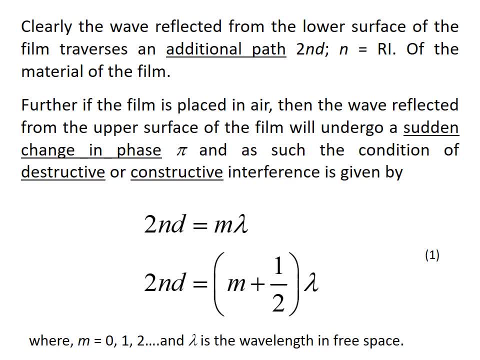 interference that we discussed earlier, that for constructive it is integral multiple of n, integral multiple of lambda, whereas for the destructive it is n plus half lambda. then, due to the phase change of pi, the constructive interference condition becomes m, m plus half lambda, where n- i am not taking n, which was taken earlier, because we will get confused with the refractive index- 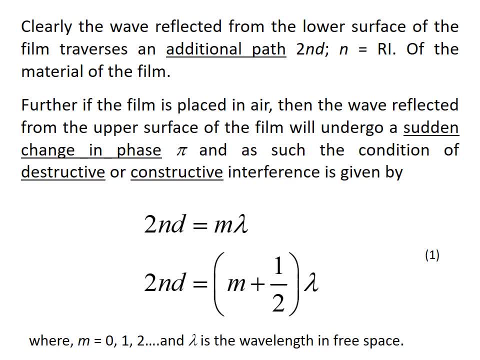 term which i am presenting by n, where m is usual: 0, 1, 2. what i want to say here is, initially, that is, the interference by the division of the wave front method. the condition of constructive interference was the part difference should be the integral multiple of lambda, for the destructive interference was 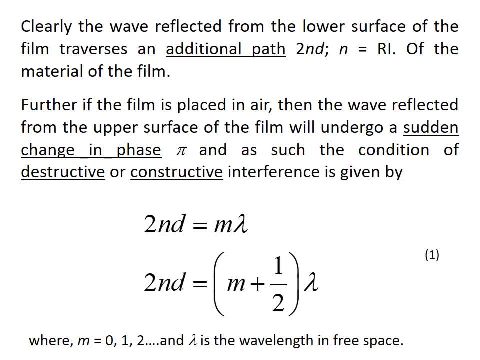 part difference should be m plus half lambda. however, due to the reflection or the phase change of pi from the upper surface because of the presence of the rarer medium, or the movement of or the air intervals of the medium, is out to To the end of our ground. i will talk just about the quantum of mysterious particles. so 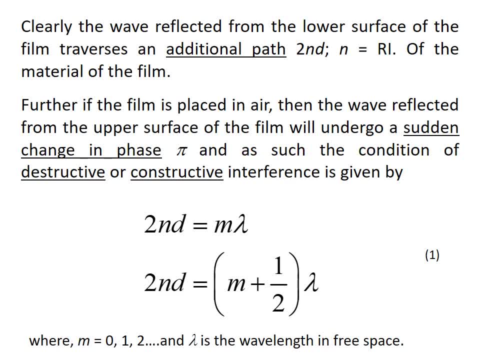 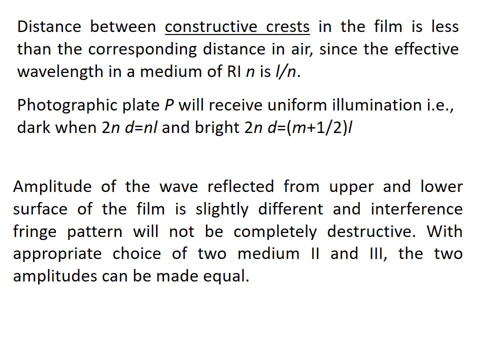 Air is going from rarer to denser medium. The conditions reverses. Now my constructive interference condition becomes 2nd. equals to m plus half lambda. The distance between the constructive crest in the film is less than the corresponding distance in air because of 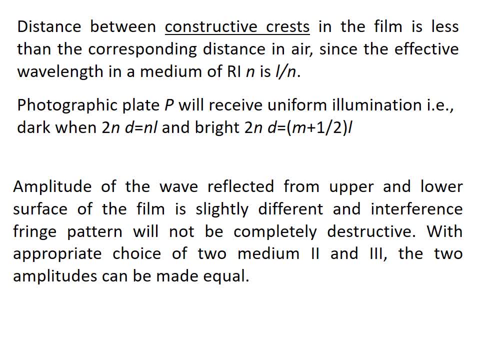 the medium as a refractive index which is more than that of the air. Therefore the wavelength becomes I by n. The photographic plate P will receive uniform illumination that is dark when 2nd equals to ni. This is the minima condition for the constructive interference. bright when 2nd equals to m plus half pi. 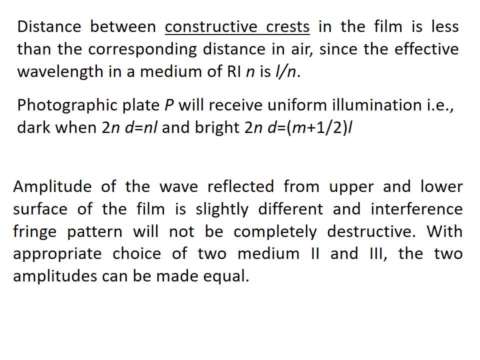 As you can see, the conditions have changed. All views are correct. What we have done here is we have replaced the value of lambda with I by n In the conditions of maxima and minima or conditions of constructive and destructive interferences. The amplitude of the wave reflected from the upper and the lower surface of the film is slightly different. 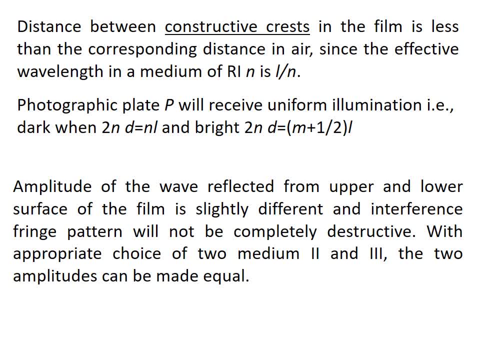 Since the amplitude, as there is a loss of amplitude, or the amplitude that you get after the reflection from the upper and the lower is different. Therefore, the interference fringe pattern will not be completely destructive, That is, the complete cancellation of amplitude does not take place. 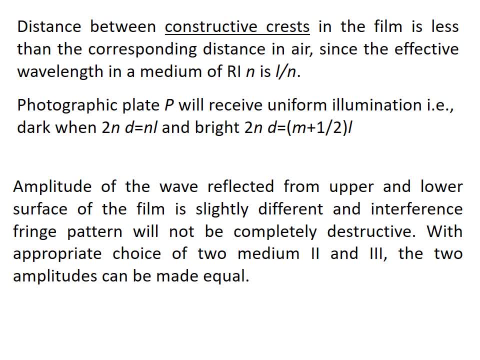 It will not be very dark, as was the case in the double slit experiment, With appropriate choice of two medium, that is, 2nd and 3rd. reference to the first figure, Figure 1 and figure 2.. The two amplitudes can be made equal. 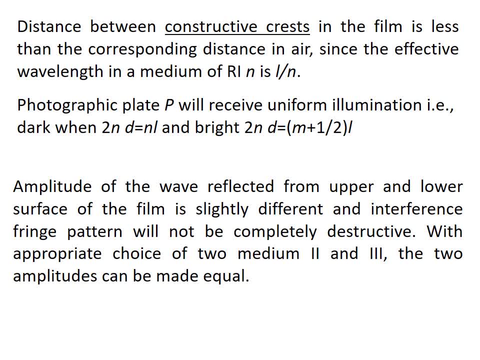 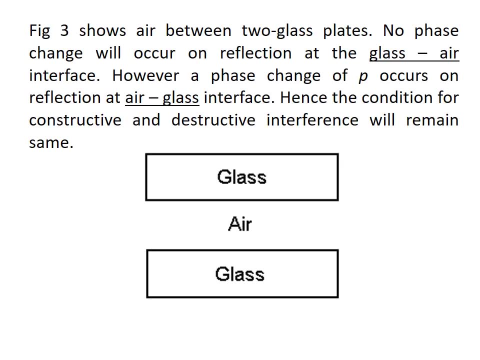 And this leads to when the air between the two glass plate is taken, Then the no phase change will occur on reflection at the glass air surface. However, phase change of pi occurs on the reflection at the air glass surface. Hence the condition for the constructive and the destructive interference. they remain same. 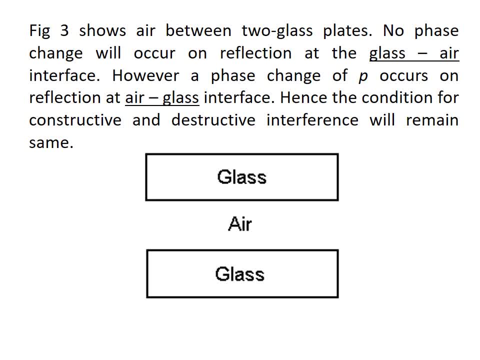 Then this is the system As in the figure here. if I take the system such as glass- air glass instead of air glass- Then the conditions which got changed due to the reflection or introduction of the pi Or the introduction of the part difference lambda by 2.. 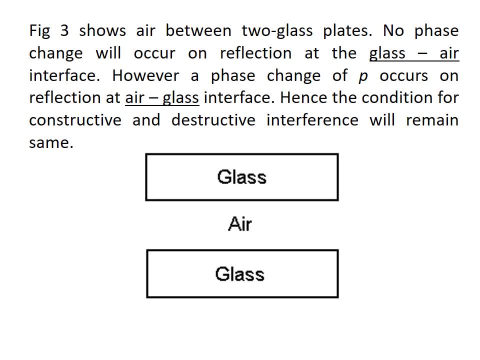 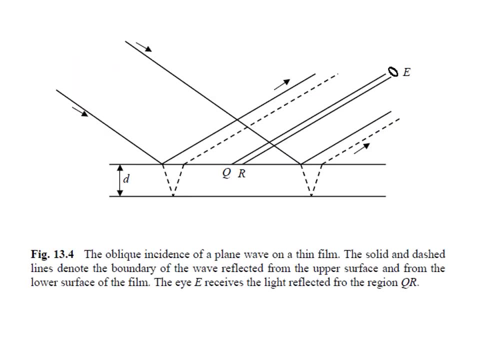 This will not occur and the maximum and minimum conditions will be same As they were in the case of division of bay front. This figure represents how the division of amplitude leads to the interference In case of oblique incidence, whereas earlier we were discussing about the normal incidence of a plane wave on a thin film. 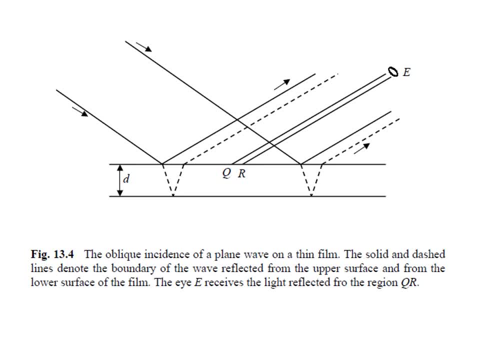 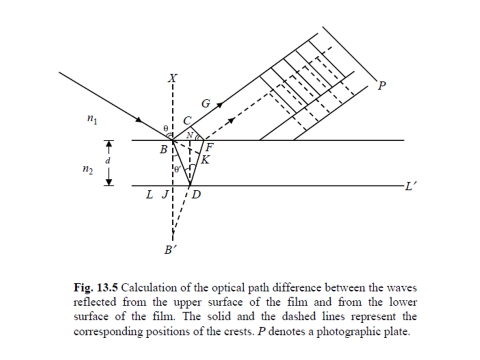 Solid line, they represent the wave reflected from the upper surface. The dash line represent the wave reflected from the lower surface. The solid line and the dash line, They somewhere interfere and form the interference pattern. This figure represents the mathematic formulation Which denotes that if the refractive index of the medium one is n1.. 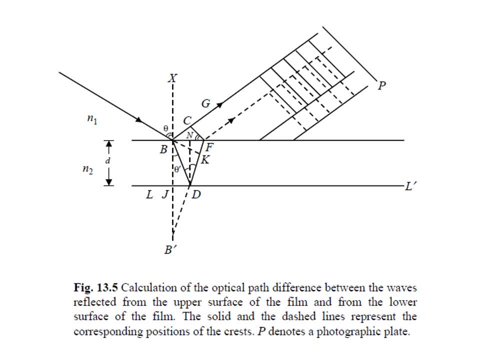 And the refractive index of the film is n2.. And the thickness of the film is small d. Then what will be my part difference? For the normal incidence case- We simply took part- difference equals to 2 nd. However, for the oblique incidence, this will not be the case. 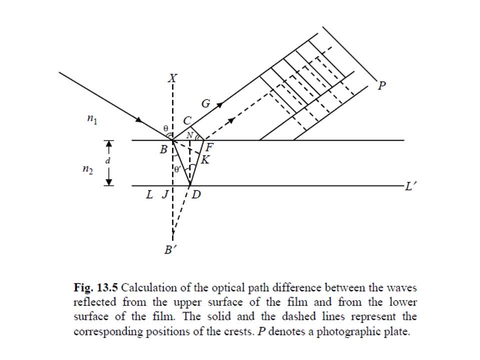 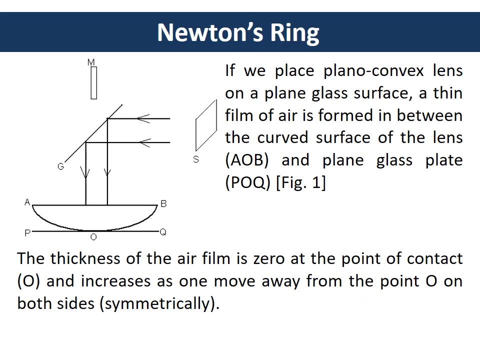 It will depend upon the angle of incidence as well as the angle of refraction. Otherwise, all the process is the same. Newton's ring is one such phenomena, Which is observed When the interference due to the division of amplitude takes place. This was named after Isaac Newton. 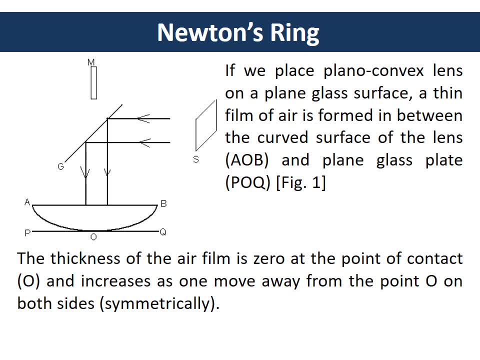 Who first observed this phenomena in 1704.. If we place a plane of convex lens that is AOB- See in the figure- A thin film of air is formed in between the curved surface of the lens that is AOB and POQ. 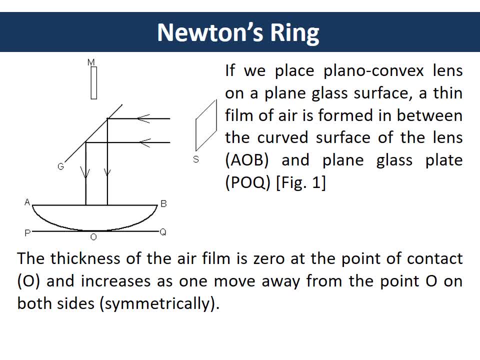 Which is the plane glass surface. This thin air film has a thickness which is not equal. It increases as one moves away from the point O And at point O its thickness is zero. One thing is to be observed is this thickness increases symmetrically on both the sides. 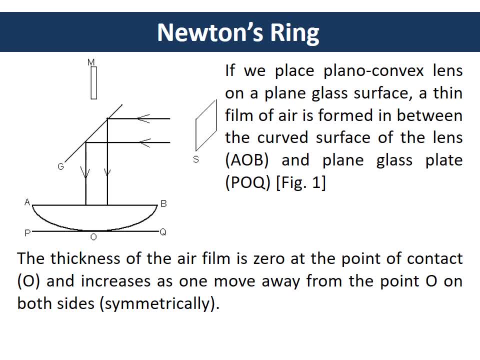 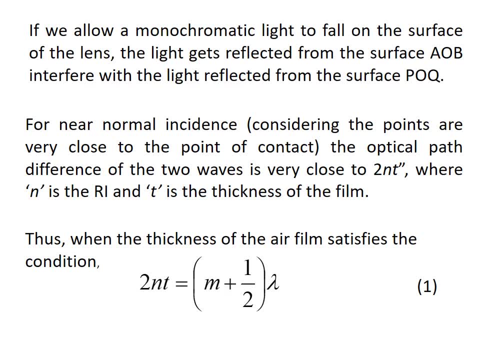 In order to obtain Newton's ring In the set up. If we allow a monochromatic light to fall on the surface of the lens, Then the light gets reflected from the upper surface Or the surface AOB. 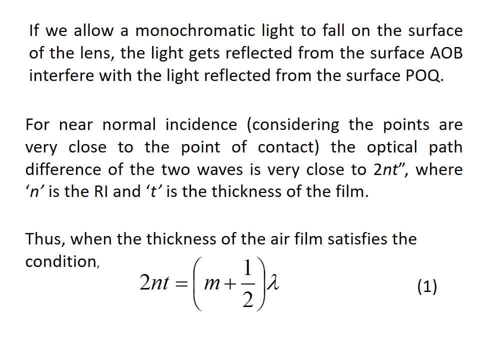 And interfere with the light reflected from the surface POQ, Which is the surface of the plane mirror. Now for the rear. considering the points are very close to the point of contact the optical power difference of the two waves. it will be very close to 2 NT. we are taking the 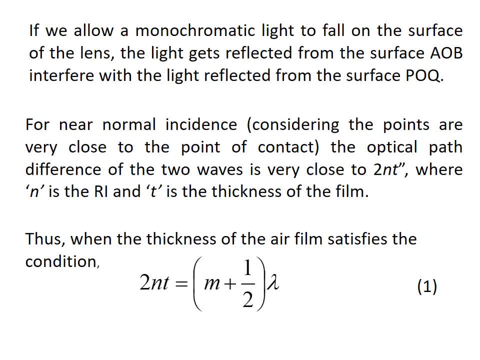 approximation here, if it is the case of normal incidence, where N is the refractive index and T is the thickness of the air film. thus when the thickness of the airfcam satisfy the condition, or we can say, if the part difference is equal to n plus half lambda, then this is the condition of maxima. 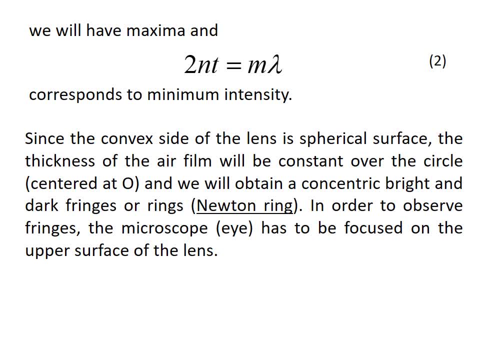 and if the part difference 2 NT equals to M lambda, then that is the condition of minimum or corresponds to minimum intensity. since the convex area of the fiber is very compact and the incidence of the air film is very of the lens is a spherical surface. the thickness of the air film will be constant over the circle. 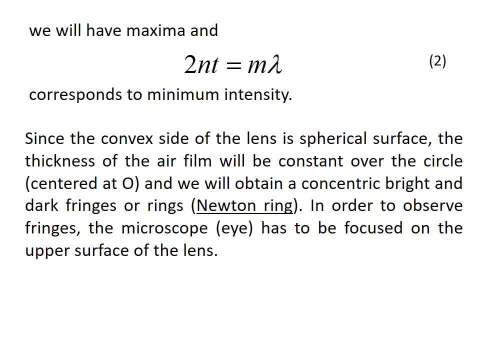 that is, it is symmetrical on full ring, centered at o, and we will obtain the concentric, bright and the dark fringes, or the rings these construct. concentric, bright and dark fringes are known as newton's ring name after newton, isaac newton. in order to observe fringes, the microscope. 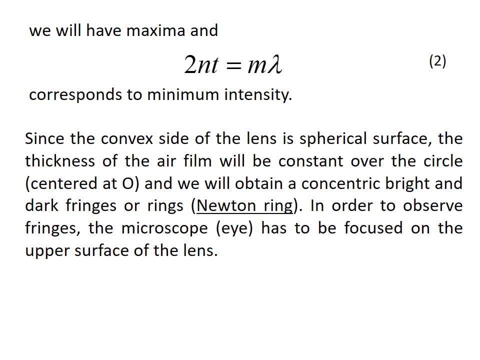 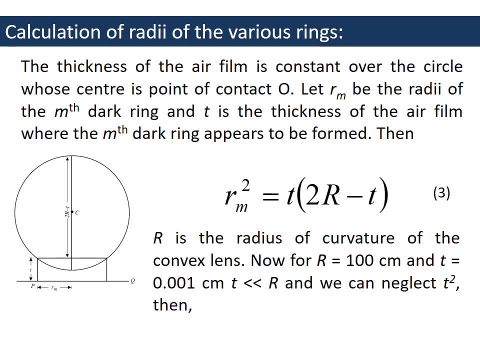 or the eye has to be focused on the upper surface of the lens. up till now, we have the condition of dark fringe and the condition of bright fringe. now we will be calculating the radii of the various rings. we know that the distance of the air film is constant over the circle. 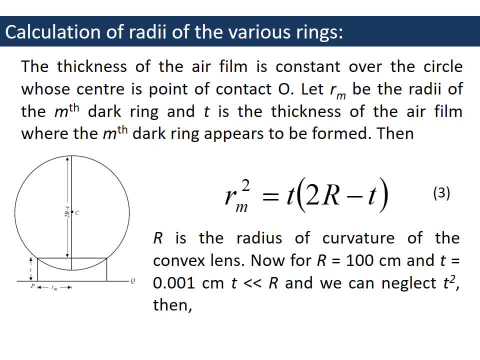 whose the the center is point of contact. o let rm be the radii of the mth dark ring and t is the thickness of the air film where the mth dark ring appears to be formed. we have the. we are finding out the radii of the mth dark ring because the condition for the dark or the dark fringe is: 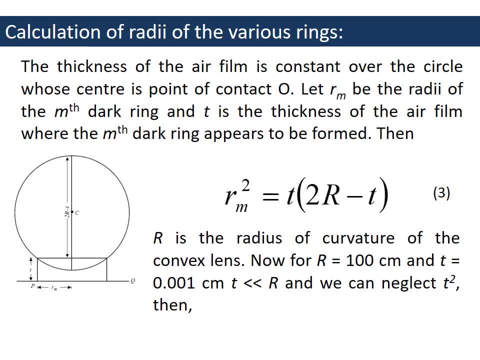 easier. that is 2nt equals to m lambda. therefore, using the properties of circle and the serval of d over Ph, o are: the rm is equal to our mth fat s equal to rm s. so we have 3 inha of V and p? t. 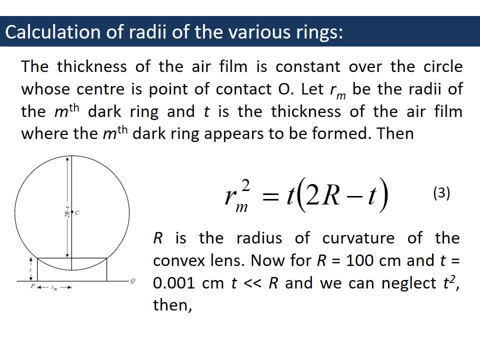 reason here into 2r minus t remaining. I am using the property of the circle, where capital R is the radius of the curvature of the convex lens. Now my r is 100 centimeter and my thickness of the air film is around 0.001 centimeter, which is very, very less compared to the capital R. 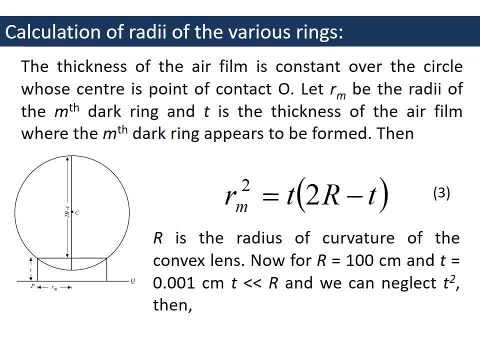 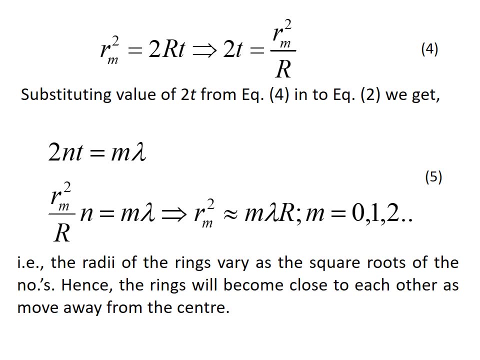 Therefore, we will be neglecting t square and my equation simplifies to rm square equals to 2rt. You get that radius of the mth ring is under root of twice rt, where my capital R is the radius of curvature of the lens. Substituting this value of 2t from the equation 4 into the equation 2, which 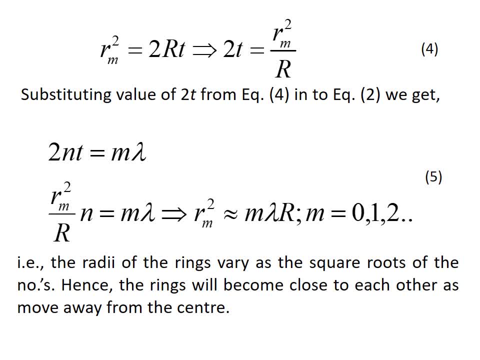 was the condition of the structure of interference. that is part difference equals to m lambda. we get that rm square is almost equals to m times lambda, capital R, where m is 012.. This means that the radii of the ring they vary as the square root of the numbers. Higher the numbers, less is, the more is the radius, Hence the rings. 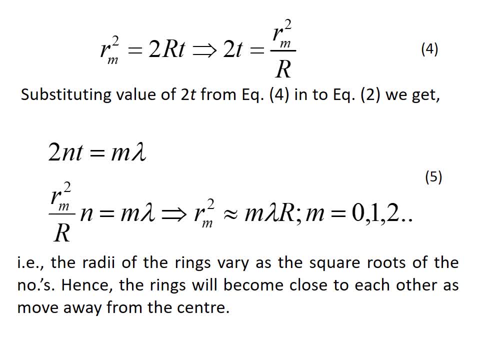 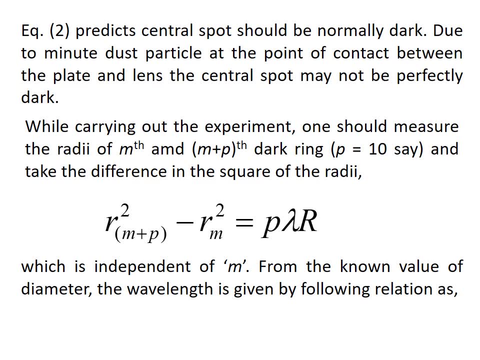 will become close to each other as they move away from the center. You can see that the centre of the explaining will be too dark and we can see that any elemental light. use the Linux, it might not be perfectly dark. while carrying out the experiment, one should measure the radii of the. 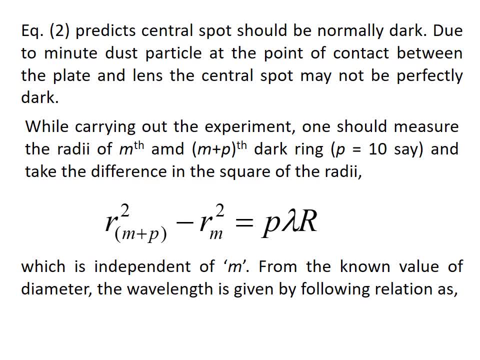 mth fringe and the m plus pth fringe, p. for example, say 10 and take the difference in the square of the radii m plus pth fringes. radii square minus mth fringe radii square equals to p lambda r, that is after calculation, which is independent of m. previously, as we were seeing that the radius 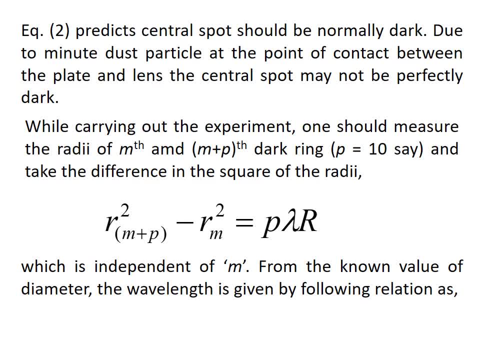 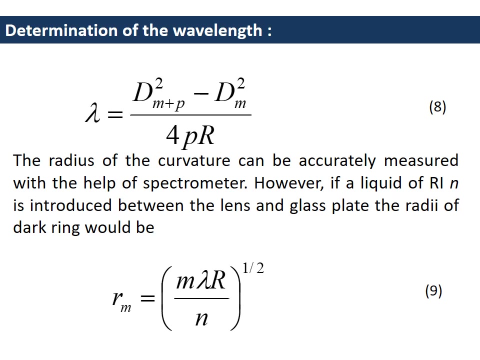 of the dark fringe is depending upon the numbers m. how, therefore, in order to eliminate the dependence of m, we have, we have used this concept from the known values of diameter. that wavelength is given by the following relation: this is in terms of the diameter, instead of the radius, of the dark fringe, diameter of the m plus. 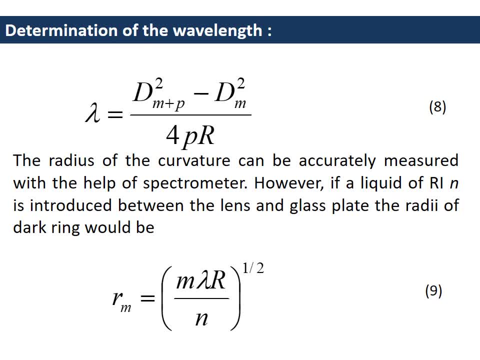 pth and the mth dark fringe, if the radius of the curvature can be accurately measured with the help of spectrometer also. however, if we introduce a liquid of the refractive index n between the lens and the glass plate, then my lambda will simply be lambda by n and the and the radius of the dark fringe changes to or reduces.